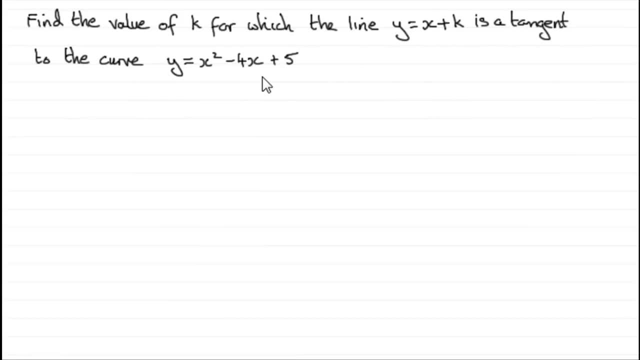 is a tangent to the curve y equals x squared minus 4x plus 5.. And to get an appreciation of this kind of question again, I would suggest you try and sketch this. So, if we were to look at our curve, the quadratic curve y equals x squared minus 4x plus 5,. 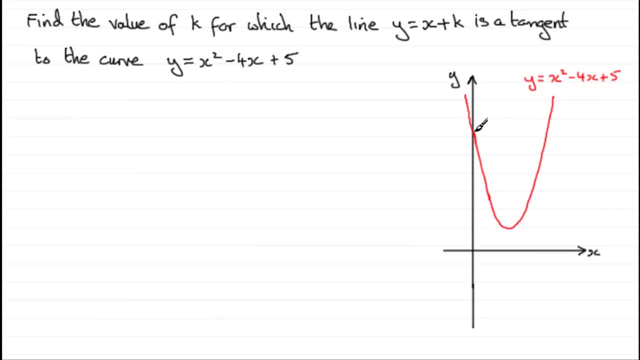 what we've got is a curve that crosses the y axis when x is 0, that will make y equal to 5.. So we just mark that in there as 5.. Now we've got our line: y equals x plus k, but we don't know what this constant k is. 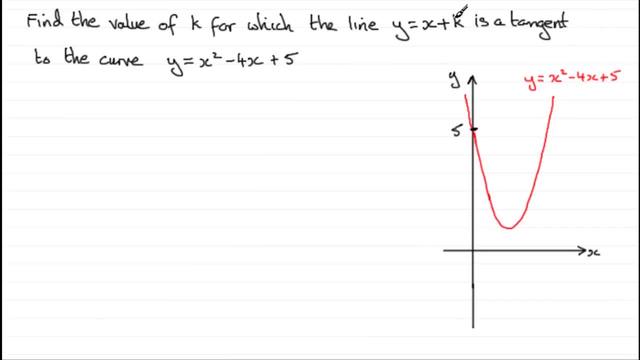 Any line of the form y equals x plus a constant is going to have a gradient here of 1, positive gradient 1, so it's going to be a line sloping up something like this. Let's just draw a general line in there you go: y equals x plus k. 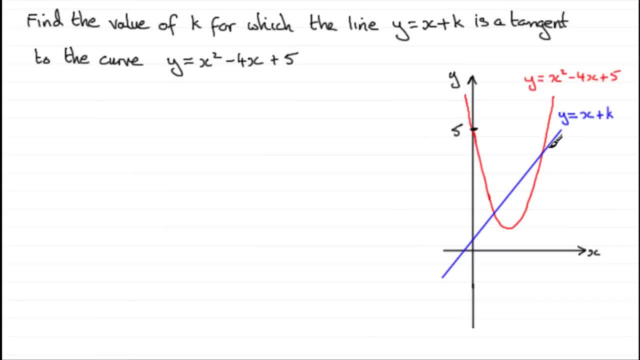 now, clearly you can see that this line is crossing the curve at two points of intersection. now, if it were a tangent, then this would happen: our line, instead of being there, would be somewhere down here. now that would mean that at this point there'd be just one point of intersection. 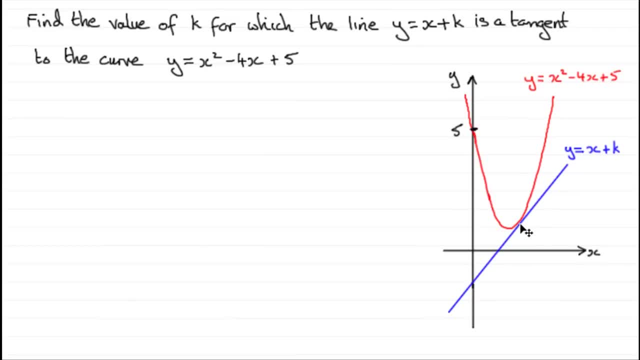 or it just touches. there'll be one root to our equation, unlike this one, two roots or, down here, no roots. so for a line to be a tangent to the curve here, then there's just got to be one root in our solution, and our solution is going to be the solution to a quadratic equation. 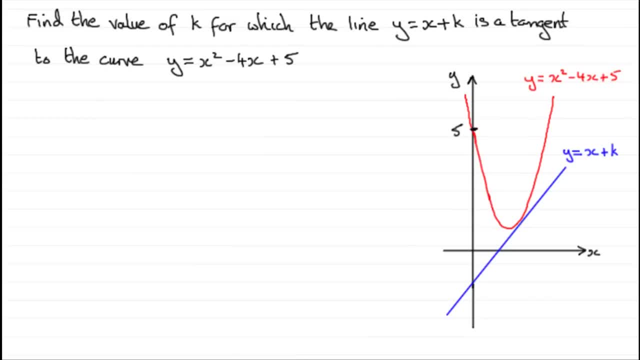 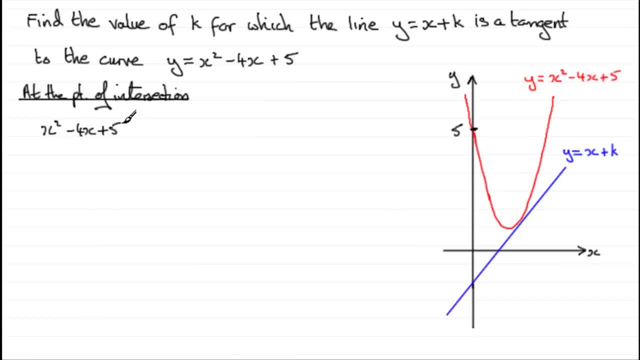 x squared minus 4x plus 5 must equal the x plus k. Alright, the y coordinates will be exactly the same at this point for some value of x. Now we've got a quadratic equation because of the x squared, so we need to rearrange it, make it equal 0.. 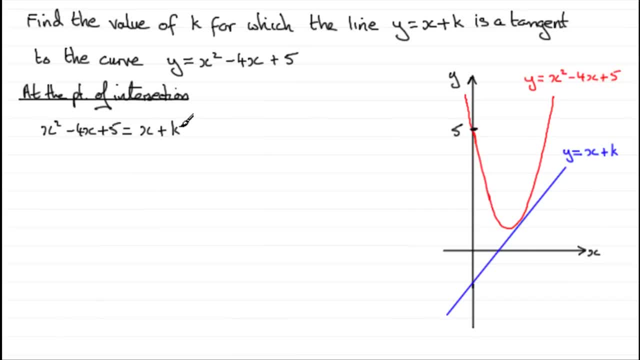 So if we subtract x from both sides and subtract k from both sides, we're going to get x squared minus 4x minus another x is going to be minus 5x, And then we've got the 5 minus the k. plus 5 minus k equals 0.. 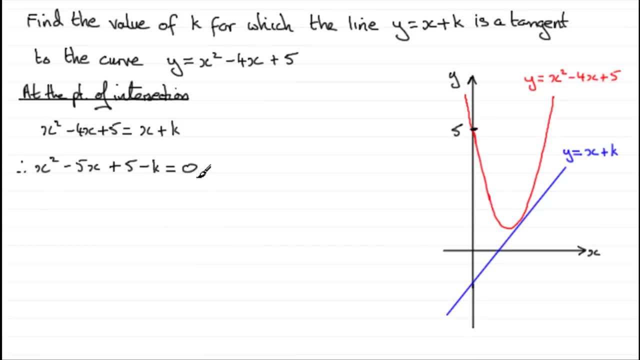 Now, when I'm doing any quadratic equation, I like to have my x squared term, then my x term and then my constant on the end here equaling 0.. Alright, But can you see that we've got two terms here which are constants, and I want to have this as one term. 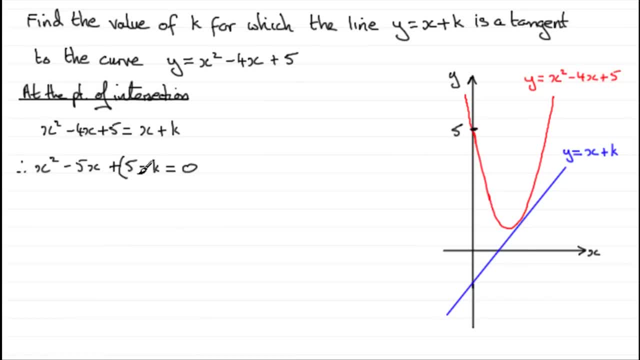 So in a case like this, what I would do is put a bracket round here. That's very straightforward, because I've got a plus here. that's going to be plus 5 minus k. But remember, if you had a minus there, you've got to be careful over the signs so that you get them to agree with the previous line above. 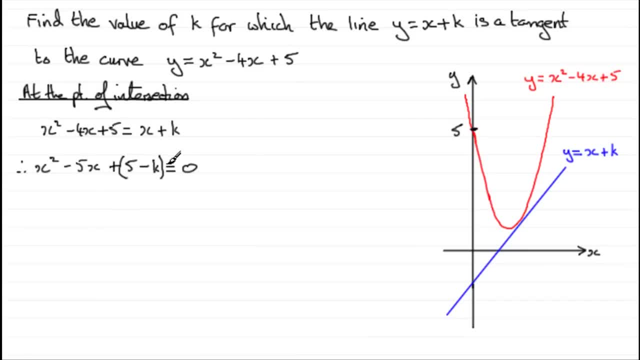 Okay, so I've got three terms here. Now this is the good bit. This is the bit where, if a line is to be a tangent, there's going to only be one root to this equation. So let's just put a little bit of info here. 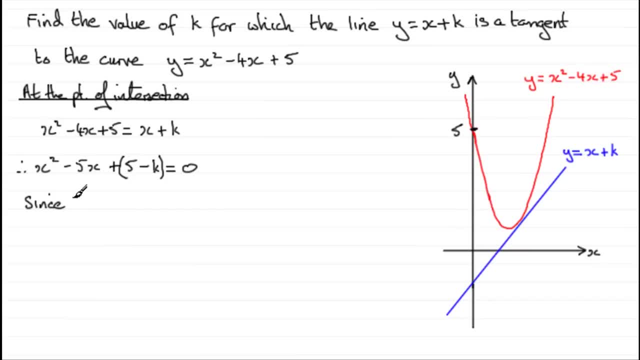 Okay. so we'll just say that, since the line is a tangent, there must be one root. There must be one root. One root, one solution, okay. So therefore we know that the discriminant in the quadratic equation, ax squared plus bx plus c, equals 0,. 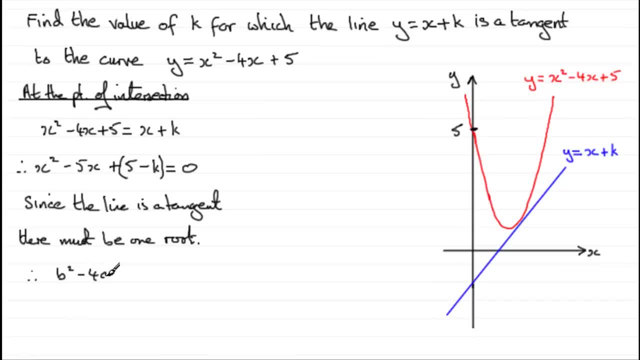 the discriminant, that is, b squared minus 4ac, must equal 0.. And what is the b value? Well, b is the minus 5.. So we've got minus 5 all squared. Let's put a, therefore, in there.